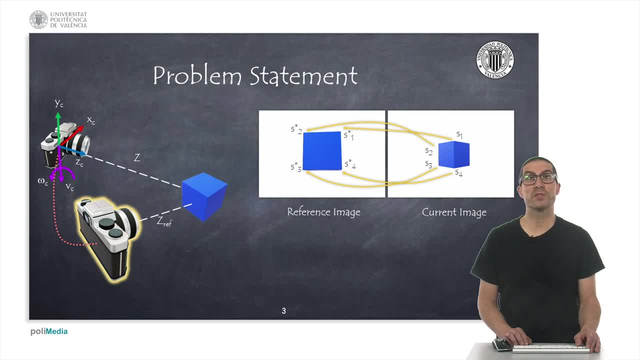 to the camera and we want to control the position of such reference frame based on its linear and angular velocities, represented here by the purple arrows. The reference of frame of the camera to be moved is represented here by the red, green and blue arrows. 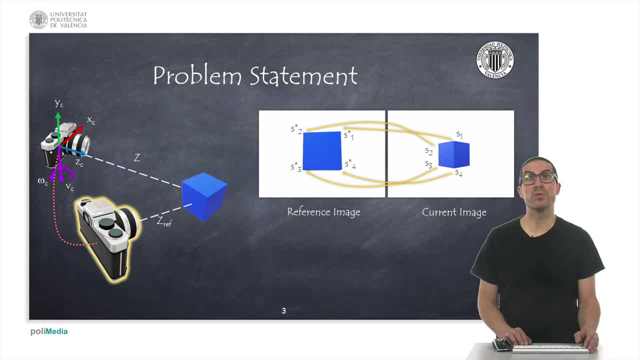 The problem to be solved consists in determining a control law to move the camera to a position so that the observed image resembles, or is identical to, a reference image. Thus, the camera can easily observe the object from a new position. However, given a reference image of that position, 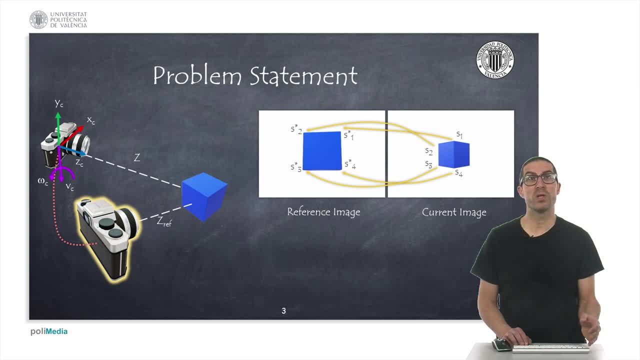 it should have been observed from other position that we don't know. So actually, this position that we don't know it is highlighted here as legendед, as subsid supervision On the by the orange border. The information that we have been provided are some points or characteristics of the image that we will associate to other points. 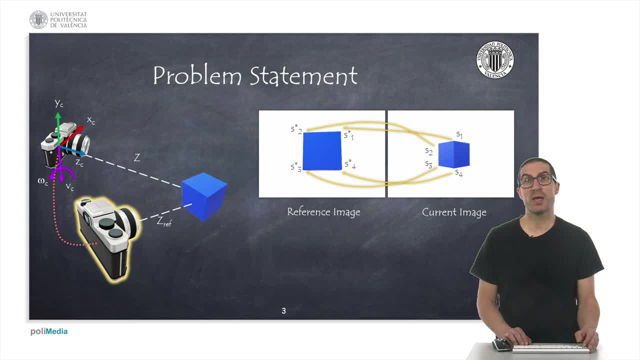 on the reference image. The difference in pixels between those points will define an error to be minimized. thus, the controller should provide a movement such that it moves the camera from our current position to the orange one. For simplicity, we will assume that we also know the depth at which the current and 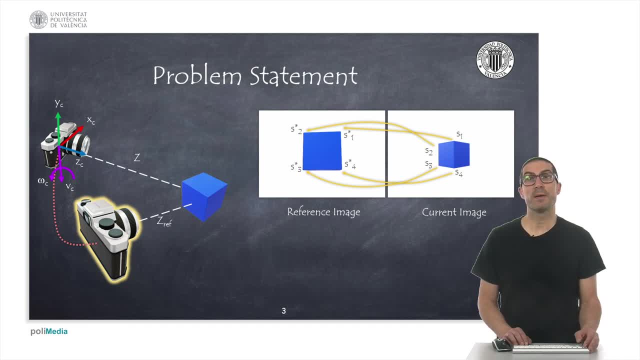 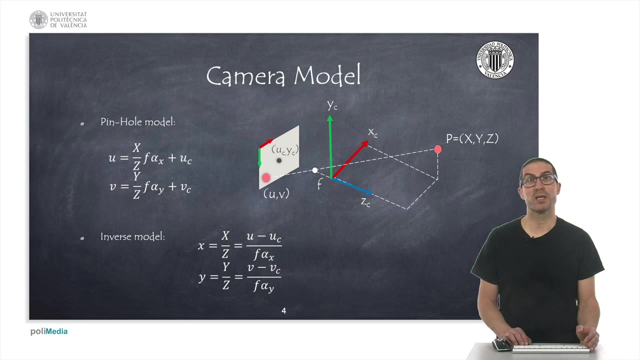 reference points are- and this is associated with the z-coordinate of the point. We will see later why we make this assumption and what it implies- A point P in a 3D space defined by its x, y and z coordinates. it. 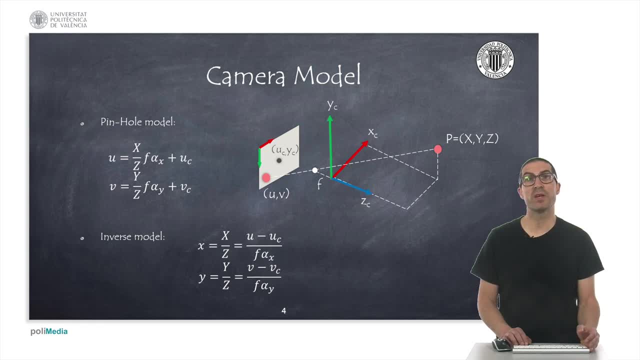 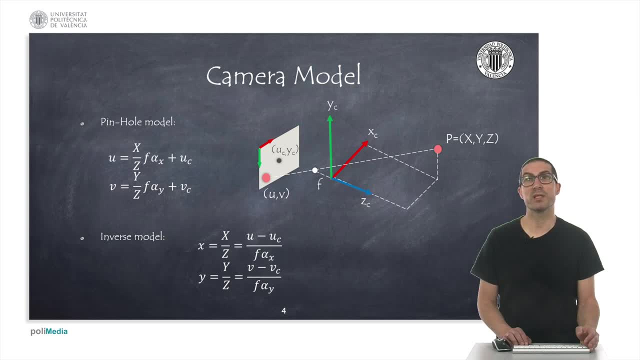 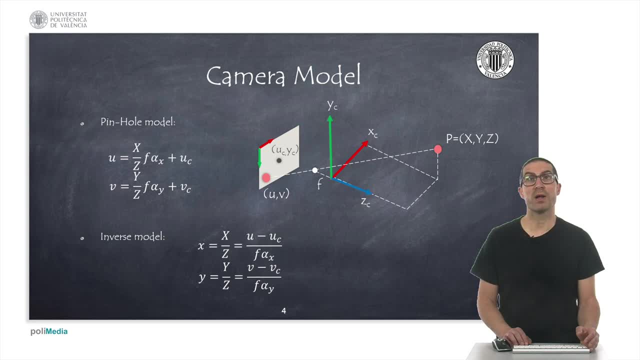 F from the coordinate system. This is the focal length. Here I have included the formulas typically used for this type of camera models, in which the intrinsic parameters of the camera are the focal length, the coordinates of the optical center, uC and yC, as well as the parameters alpha, which represent the 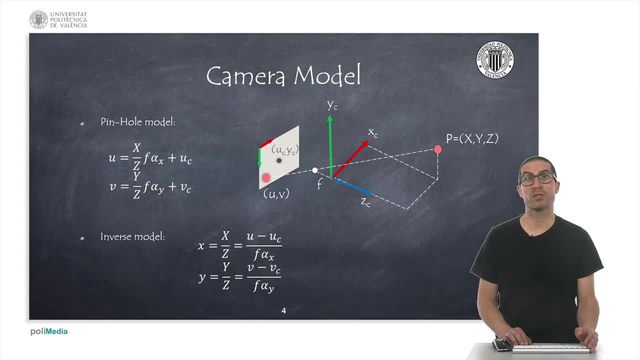 radius between the world units and pixels, pixels. This model can be used both to obtain an image point from the 3D point and vice versa, That is, from an image point we can obtain the x and y coordinates of a homogeneous point. that is a point that depends on the depth. that will 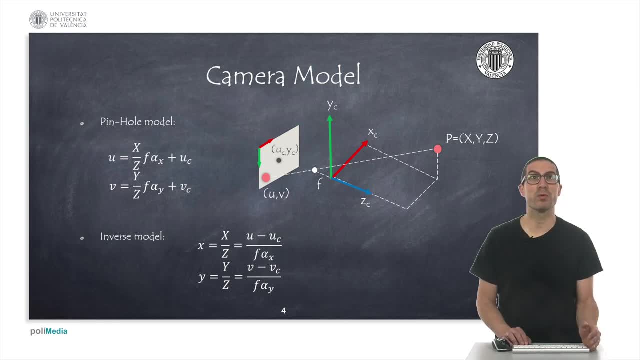 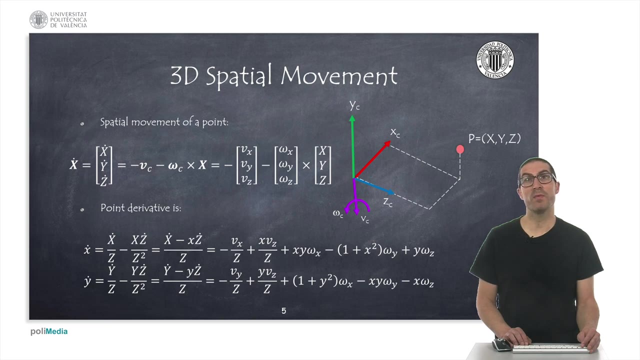 be provided in a different coordinate, so this depth will provide different coordinate values. We will consider these homogeneous points as if they were the points on the image, since they are obtained from them. Now, if the camera's reference frame moves with a linear velocity- vz- and an angular velocity, 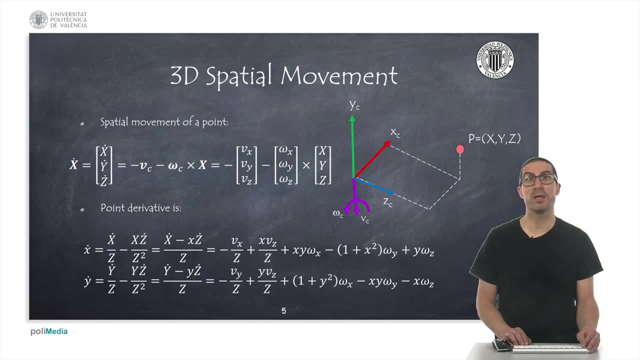 omega z, then the coordinates of the point P with respect to the camera frame itself acquire velocity, The expression I show here. it is actually a well-known expression in 3D spatial movement and it reminds the speed of the camera to the point that it is observed from the camera's reference. 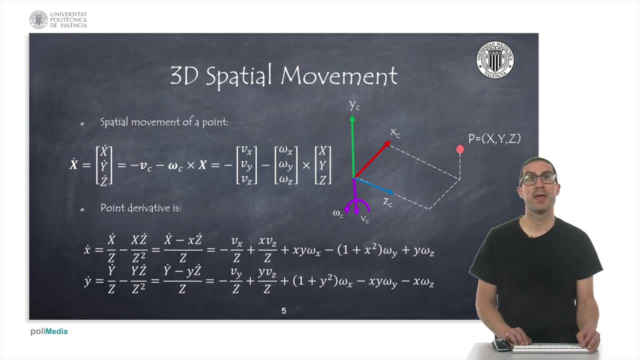 frame moving at a certain linear and angular velocities. Therefore, these speeds will be observed in the image as the derivatives of the homogeneous points, as indicated here. As it can be seen, they have a linear relationship with respect to the linear and angular velocities of the reference frame. 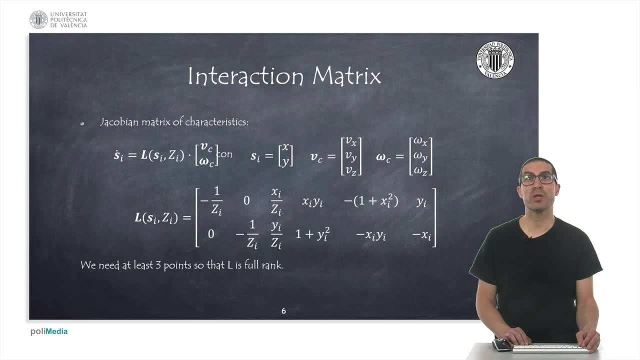 Therefore, we can express the homogeneous coordinates as a linear relationship, obtaining a Jacobian model. This is the Jacobian matrix, also known in the field of visual feedback control as interaction matrix. For each point of the image I, we will have actually a Jacobian matrix of two rows. 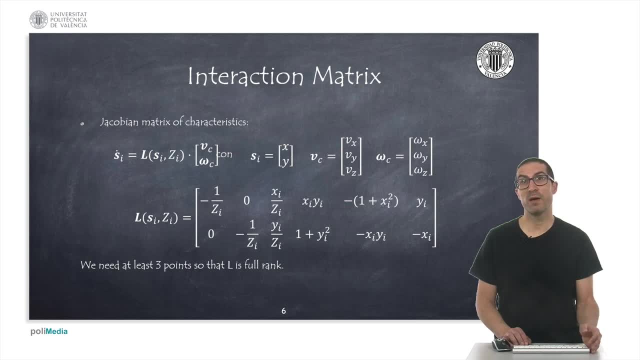 and six columns relating those velocities, the velocities of the point, with the linear and angular velocities of the camera. This expression depends on the coordinates of the point, but also on its depth. This is something that we will discuss later. In any case, it's worth mentioning that for the Jacobian, 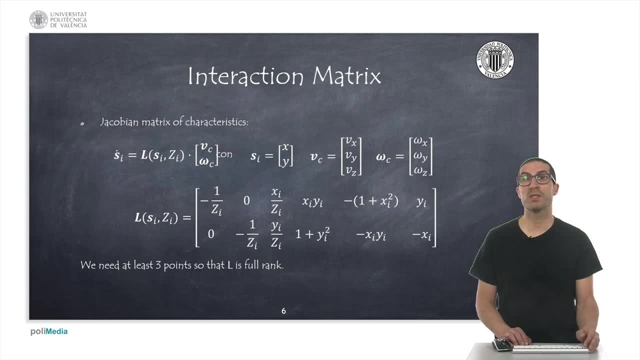 matrix. to be a full rank matrix, we need at least three points, otherwise the problem is redundant, which means that we might have multiple solutions, While if we have more points, more than three- then the problem will become a regression problem, since 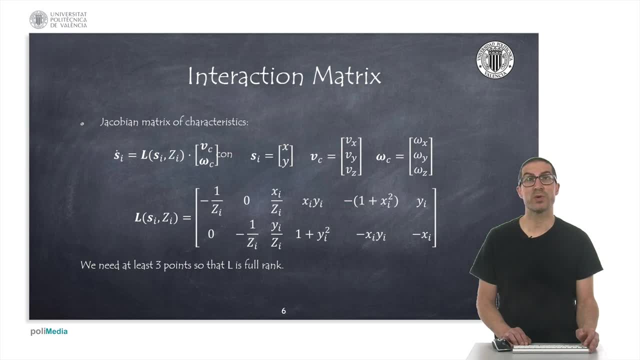 we will not be able to establish a movement satisfying all restrictions except, obviously, in an ideal world without noise and perfect models. of course, This is one of the most common scenarios. to use more points, more than three points, As already mentioned, the interaction. 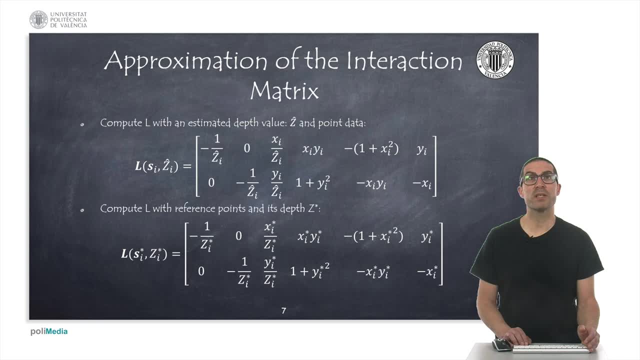 matrix depends on the point's depth. This value must be estimated. since it's a priori, we don't know this value. In any case, two approximations are usually considered. In the first one, the observed coordinates of the image and depth estimation of those. 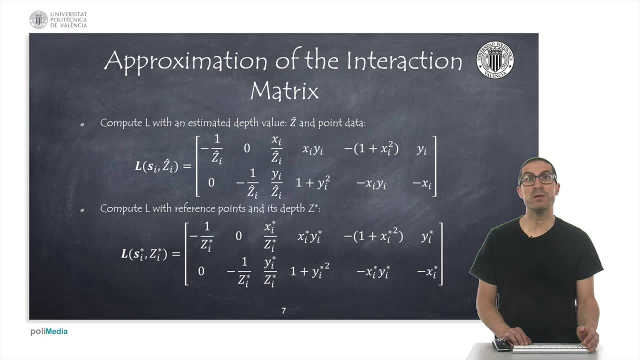 points is considered. In the second scenario, the coordinates of the reference points and their depth are considered instead. The second approximation has the main advantage that the interaction matrix is a constant matrix as long as the reference point remains unchanged. However, a frequently used approximation is to use the mean. 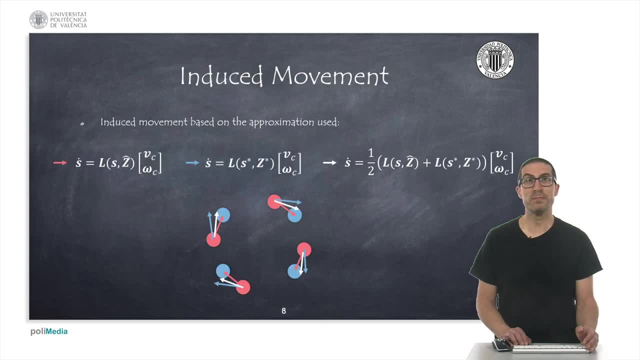 of both approximations, as we will see, The movement induced in the image plane of a pure rotation by using the characteristics detected on the image. using the first expression implies linear correction, which is represented by the movement that red points have towards the blue ones, with 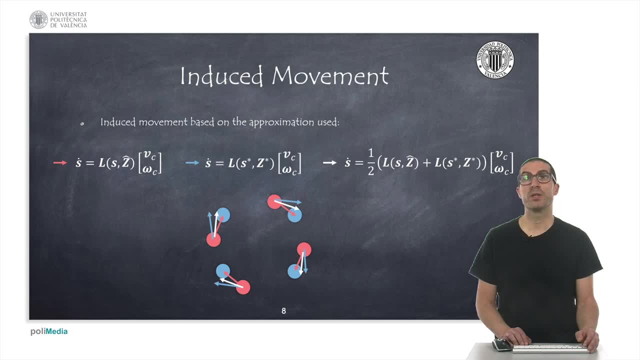 the arrows in red. On the other hand, it can be seen that, in a similar way, the movement caused by the use of the second approximation is like the one expression using the blue arrows. Both movements imply that the correction will perform a displacement and a rotation. even we know already that this is. 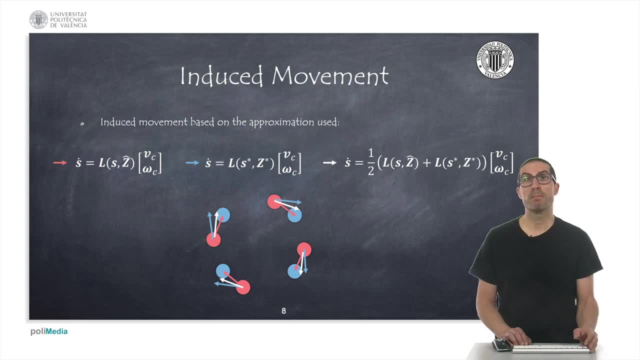 a pure rotation situation, because there's a coupling between the variables that you can see in the expression of the interaction matrix. For this reason, the mean of both approximations represented by the black- sorry, the white- arrows is usually considered a better approximation, since at least the correction 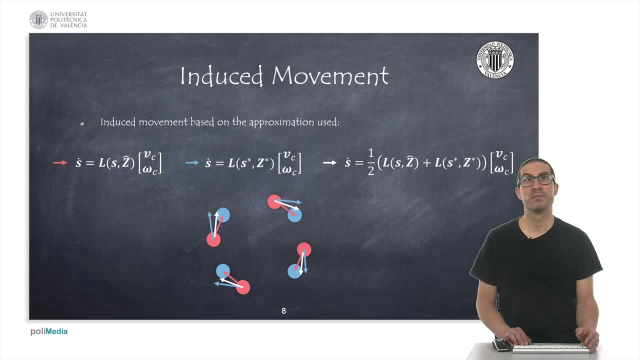 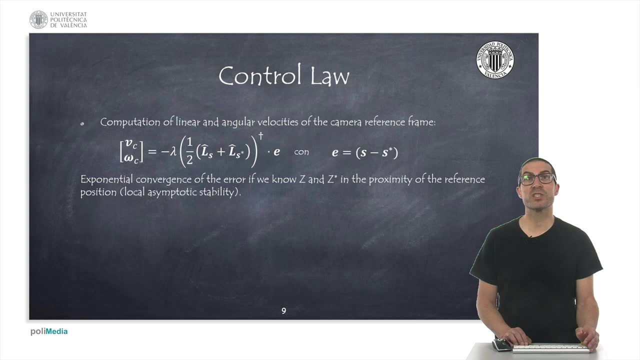 will not have the displacement component. A proportional controller on the error between the detected and reference features will allow an exponential convergence using the pseudo-inverse of the interaction matrix. The convergence is guaranteed in the proximity of the reference position. This is a local, asymptotic convergence, if we know z and z star. 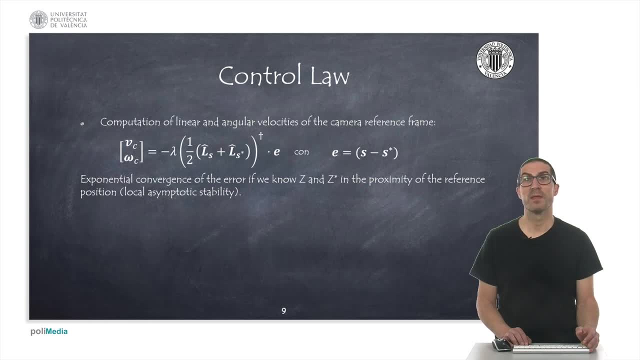 In practice the region of convergence is reasonably large. Here we have used a compact notation of the interaction matrices shown before. So the actual interaction matrix combines both the observed features and the reference features. but also the pseudo-inverse could be computed using only the observed or only 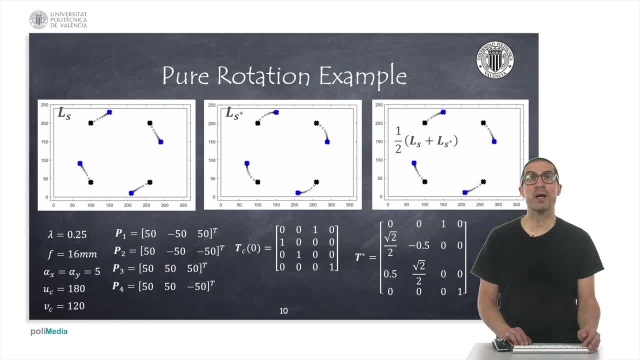 the reference features. Here I show an example with the different control proposals. Below, from left to right, I indicate the controller parameter, lambda, as well as the camera intrinsic parameters, the 3D position of four points on the initial transformation matrix of the camera's reference frame and also 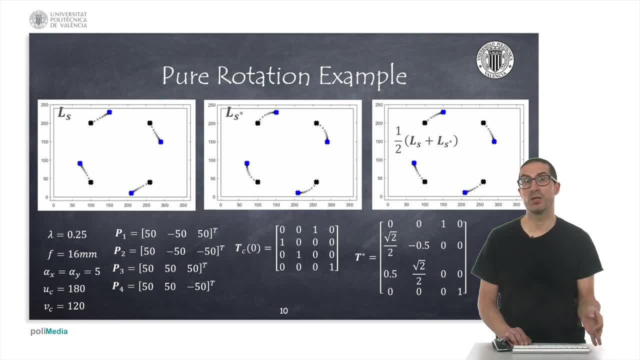 the final transformation matrix. to achieve This transformation matrix actually is used to generate the reference points on the image that are represented with the blue crosses. As you can be seen, the task consists of reaching a reference position with a rotation in the z-axis of the camera. Above, we observe three 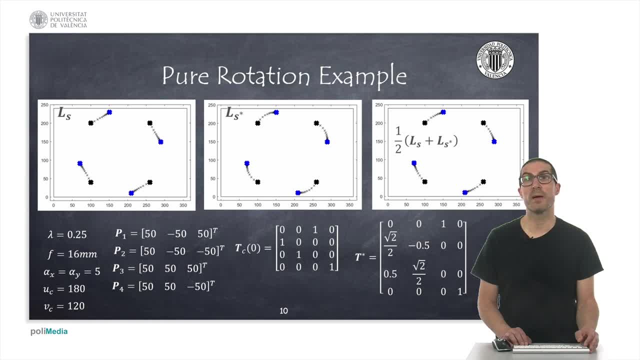 different simulations corresponding to the case in which we use the depth of the observed points with the interaction matrix LS. on the figure on the left. In the middle figure, the depth of the reference points is used with the interaction matrix LS- star, and in the image on the right we use the combination of both. It can be: